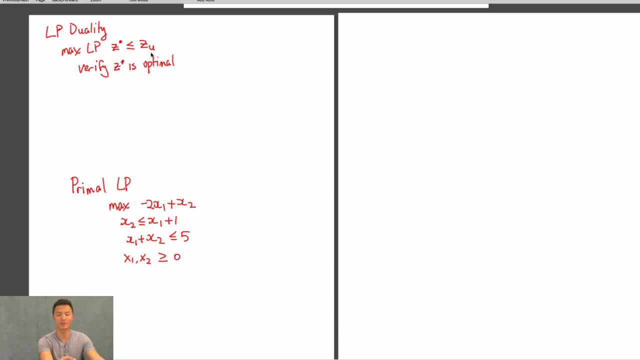 the z, because if we know the minimum upper bound of our linear program is equal to the optimal solution we found in the primal lp, then the z star has to be the optimal solution, right, Because we know that. okay, so if this is satisfied, z star is less than or equal to z of the upper bound and z of 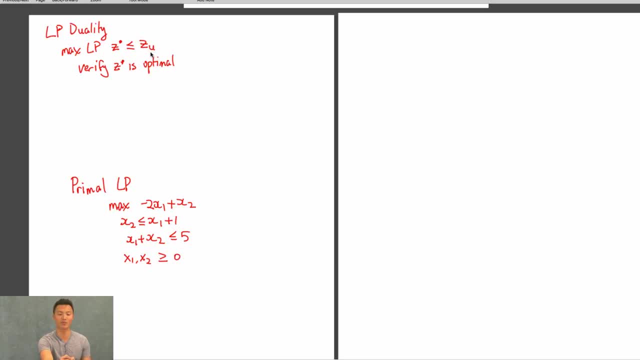 upper bound can only be the smallest upper bound is z- optimal right. If the smallest upper bound is z star, then z star has to be the. it has to be the optimal solution for the primal lp right. So we're going to define z star. 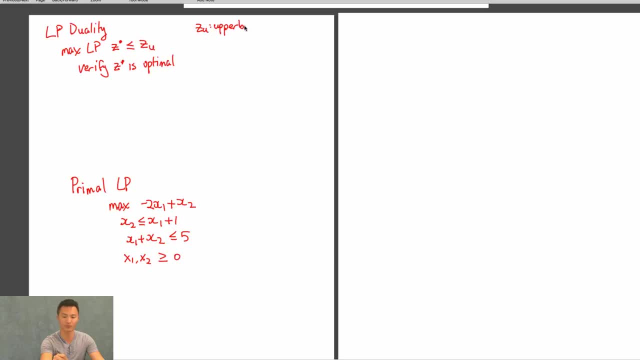 as upper bound of z. So what we're going to do here is to find some dual linear program that minimizes the, minimizes the upper bound of our objective value, right. So, objective of the dual, we're going to want to minimize upper the upper bound. 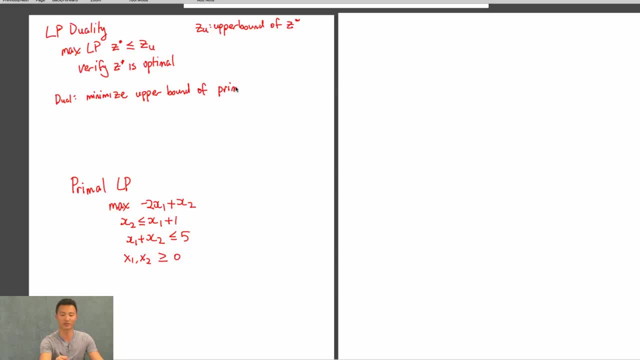 of the primal objective. If the smallest upper bound on this primal objective is the optimal solution we found, then this has to be the optimal solution, right, Because we can't go any further up, because our that's the smallest upper bound we have. 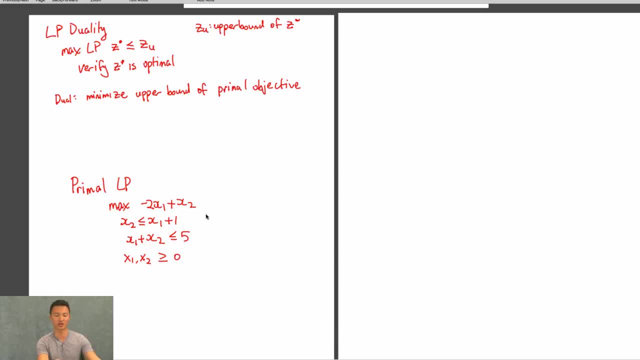 So here's an example: we have max, the objective function of negative two x one plus x two, followed by two constraints and non-negativity constraints for our decision variables. Well, the first thing we're going to do is we want to kind of generalize, put this in a general 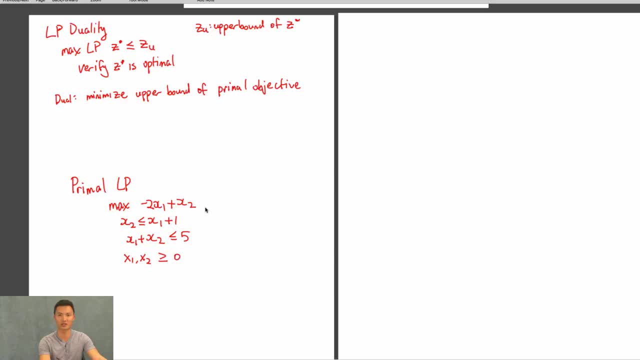 generalized format and most maximizing lp. generalization formats are going to be some equation, linear combination on the left side: less than or equal to some value, right? So in this case we're going to turn this into: x2 minus x1 is less than or equal to 1.. 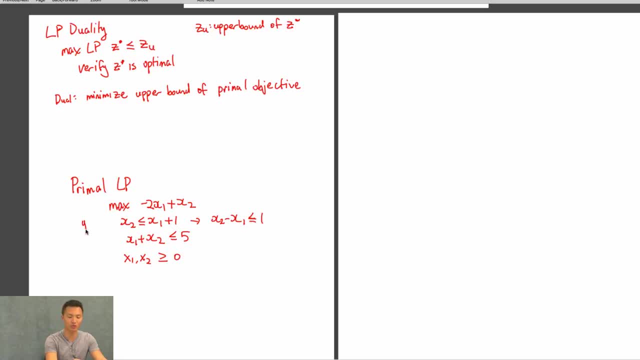 So we have our two generalized constraints. We're going to add two multipliers- y1 and y2, and we're going to multiply into the constraints and then add them up. So we're going to have y1 of x2 minus x1.. 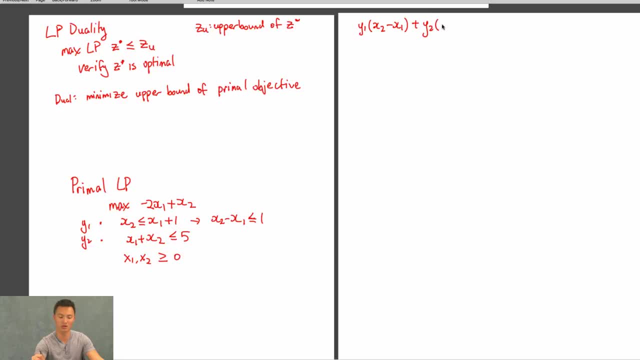 y1 plus y2 of x1 plus x2 is less than or equal to y1 plus 5y2, right. This is why we put it in a generalized format is because I can take the linear combination of the multipliers and the constraints. 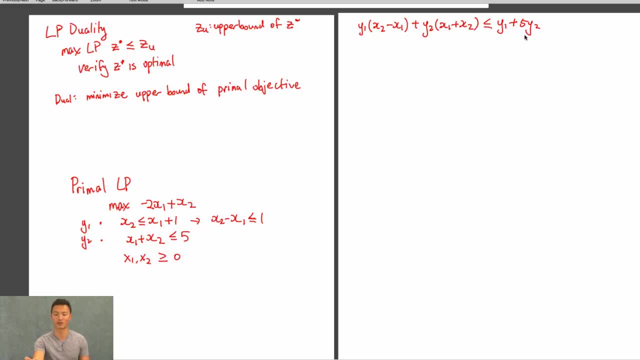 and it has to be less than or equal to the multipliers, with the constraint on the right-hand side. Well, let's think about this. Remember that we want. We wanted to find an upper bound for our objective value, right? So let's see. 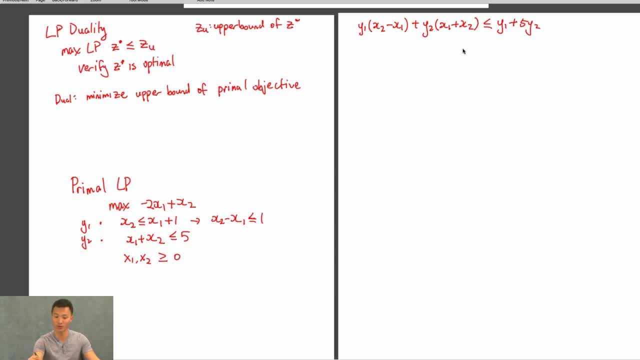 Let me rewrite this in terms of x1 and x2.. So we're going to have negative x1 plus y2 of x1 plus the y1 plus y2 of x2.. So we're going to put in equal to x1 plus y2 of x2 and y2 of x1 plus x2, of x1 plus y2 of x1. 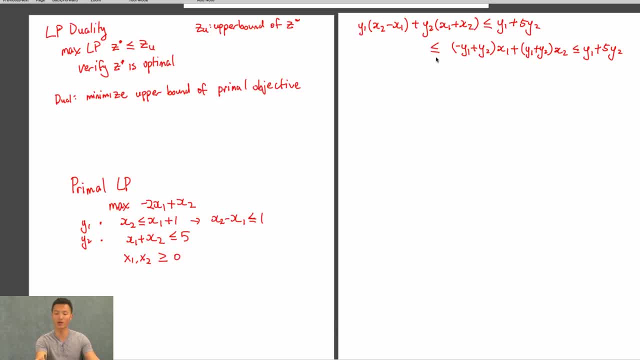 Okay, so in this dual, remember that we wanted to put an upper bound of our original objective function, which is this: negative 2x1 plus x2, right? So now we have this inequality: Our original objective function is upper bounded by this new objective function of our dual. 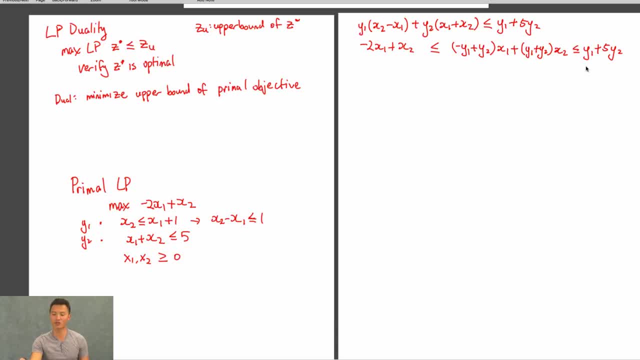 But okay, let's think about this, right, this. we need to make it so that our constraints- because originally we had these coefficients right and we don't want to use this objective value in our lp- then how do we have, like, how do we get? 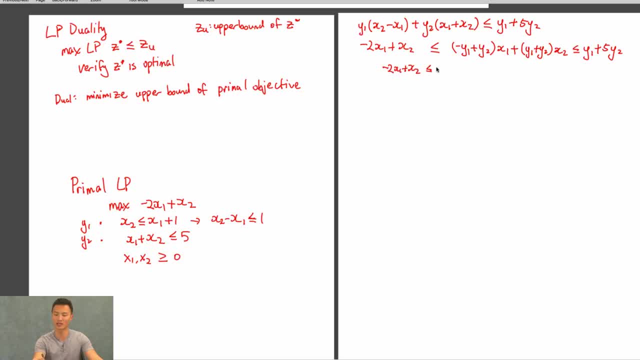 2 negative 1. x plus x2 is less than or equal to y1 plus 5y2. well, we can get it from this side right. so you see how we. i rewrote my linear combination of the multipliers and constraints into some form. 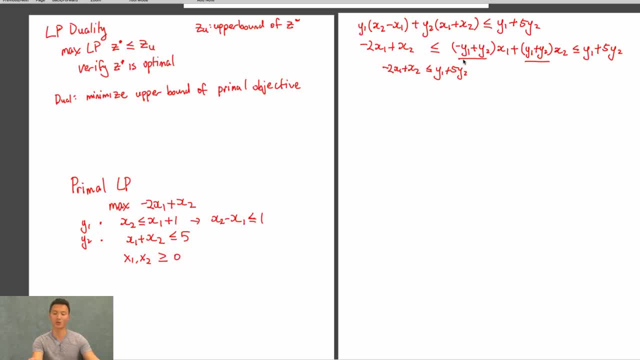 that looks like the objective function right, so this should be like: this is the coefficient of my x1 and this is the coefficient of my x2. well, we know that the original objective of the primal is negative. 2 and 1, those are the coefficients. so i want to now make these values. 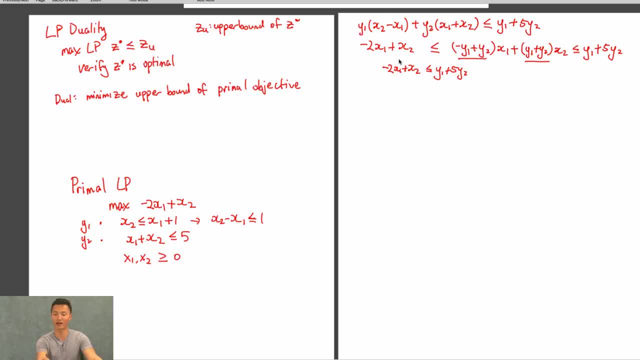 you like. i want this inequality here to hold right. i want this objective value here and this linear combination function, this inequality to hold. so for this to hold, i can set: y1 plus y2 is greater than equal to negative 2, and then y1 plus y2 is greater than equal to 1. now, by having these two, 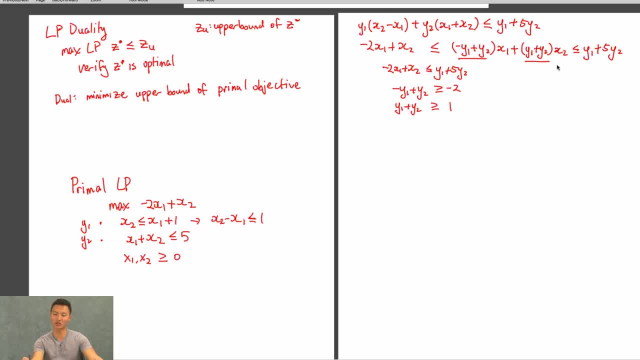 constraints, this inequality up to this point is going to hold right, and what we're going to do now is that, because this inequality holds, then i know this can be an upper bound on my primal objective function. thus, remember, we wanted to find the smallest upper bound to our objective function, and that is the set should be the same as our objective. 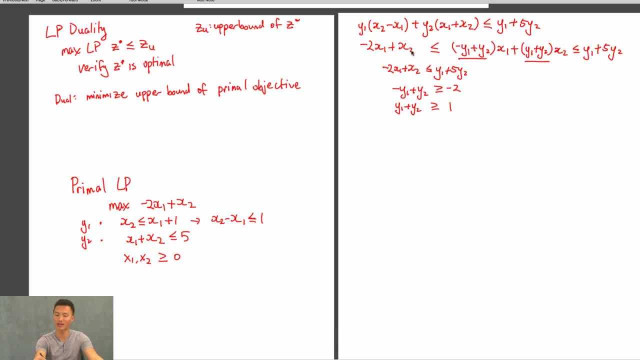 the optimal objective value, right? so let's take this: um, let's write my dual lp, so my dual is going to be minimizing the upper bound. we have right, we're going to minimize this upper bound, y1 plus 5y2, and we're going to have constraints, and the two constraints that we have. 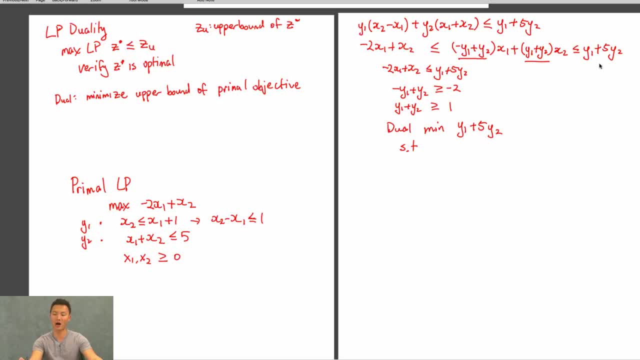 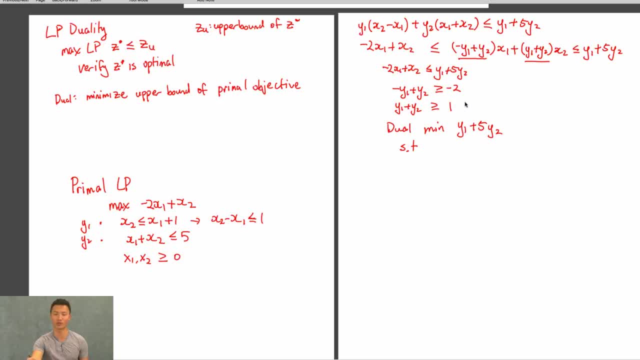 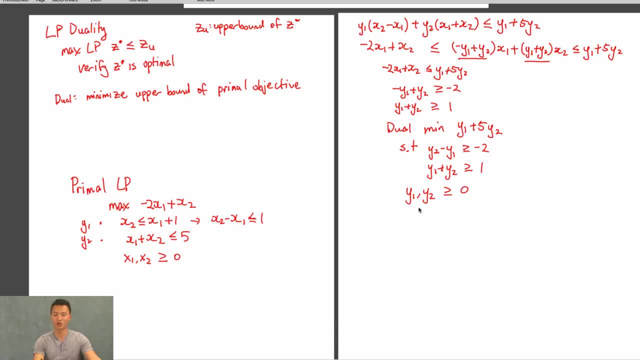 non-negativity constraints. so we need our multipliers to be non-negative, because these were inequalities, right? if y1 and y? if y1 became negative 1, then my inequality is going to be negative. so we're going to have a constant and we don't have um, we don't have our original. 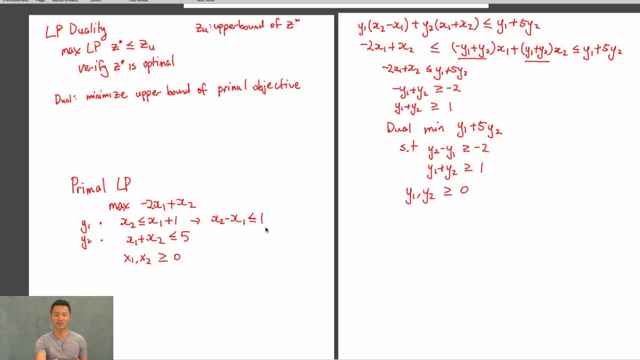 constraints back. we want it because our upper bound is basically saying that, okay, given these constraints, how can we upper bound our primal objective? now, if one of these values or both of them became negative, then our constraints change and that's not like, that's not going to. 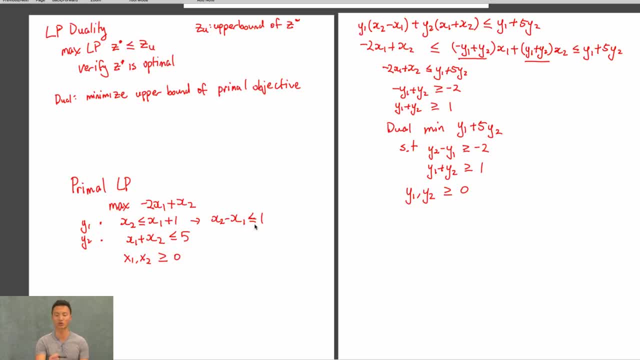 be able to tell us what's the upper bound of our objective. function value is subject to the constraints we have originally, so that's why we need the y1 and y2 non-negligent constraints, right? So let's say okay. 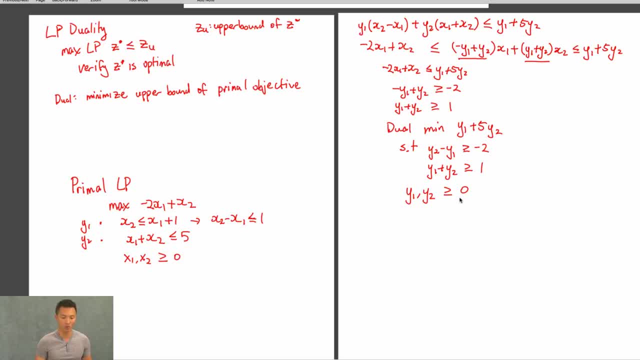 so let's say we want to solve this linear program. So one way to solve it is to just graph it out and find the two. so let's graph this out, Find the, take the points right. So we have x1 here, x2 here. 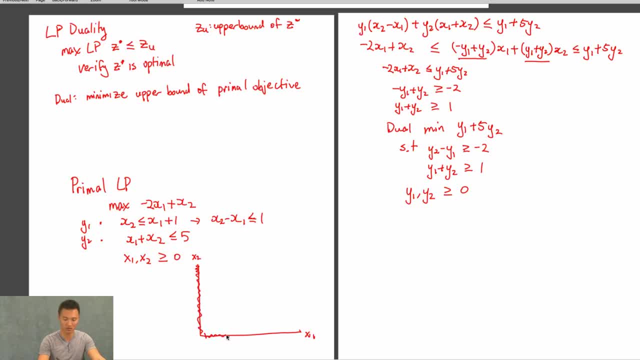 So we have the non-negligent constraints Over here And let's graph out my- what do you call it? Let's graph out my constraints, one at a time. So constraint one is going to be, let's see y2 minus one plus. 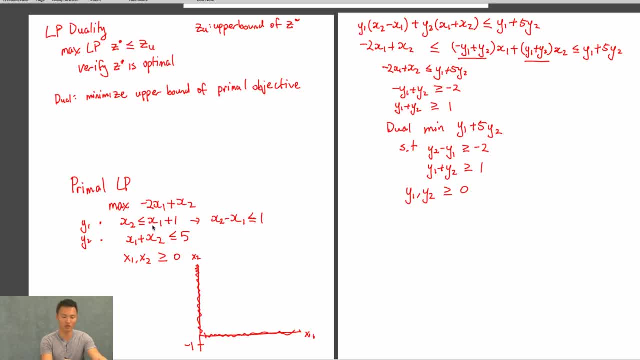 so here it's going to be negative one. Our slope is going to be one, So this is going to be one And this is going to be my, my constraint one. I'm just rewriting this inequality into slope intercept form. So we have: y2 is equal to one minus. 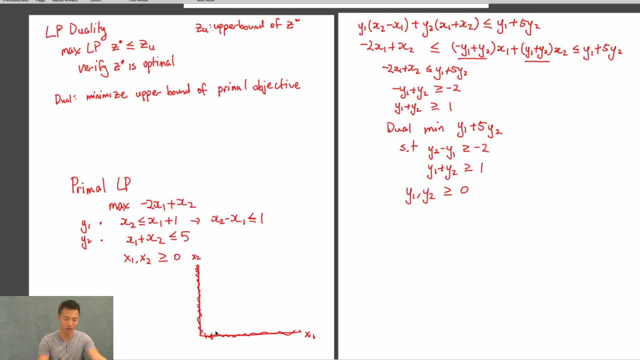 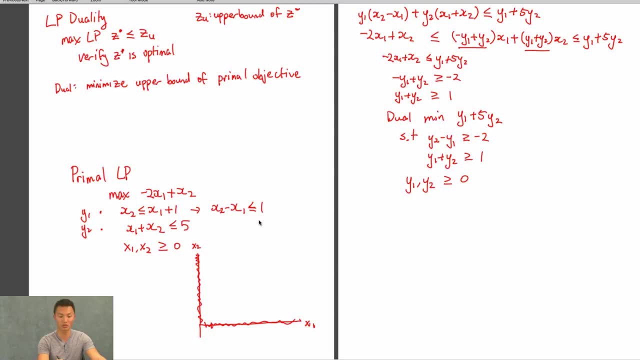 oh, whoops, Actually. okay, So if y2 is equal to y1 plus one, yeah, so actually this should be one here, And now we're going to have a slope intercept. okay, One going upwards, And this is my first constraint. 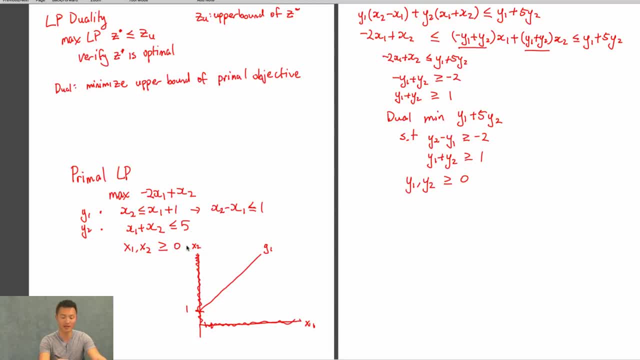 And for the second constraint we have, y2 is equal to five minus x1.. So two, three, four, five- This is going to be five over here, And I'm just going to draw this line out here. Okay, So let's see. 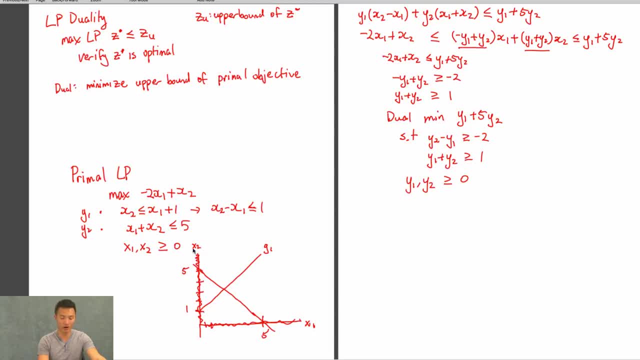 And the first constraint, if we are, let's say this is one and one, two, three. one and three, three is not less than or equal to one plus one, So we're actually going to have this region and this for our inequality constraint on g of one. 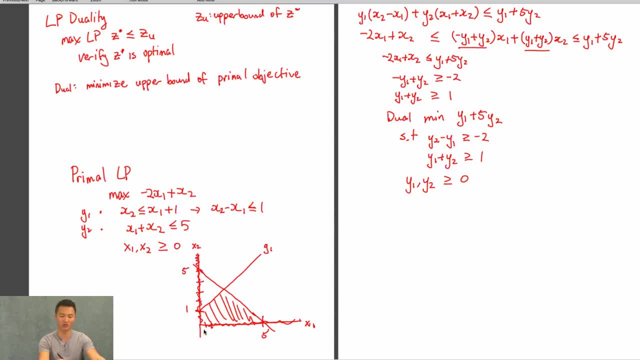 And on this side, we know that zero and zero. we check whether the origin is less than or equal to five, which it is. So everything on this side of the origin is going to equal to. it's going to be. it's going to be my feasible region, right? 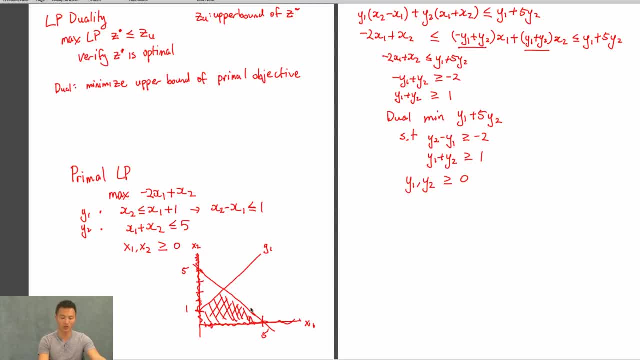 So it's this side plus this side as well. So now I have this feasible region over here and our extreme points are going to be these five: right: The linear program, the optimal value in a linear program is going to be the tangent. 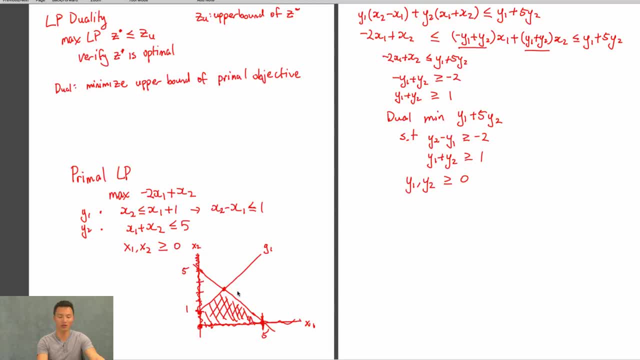 We're going to take a contour line of our objective and it has to be tangent to the extreme point, Otherwise you can just check all of these and see where it is, But I'm going to actually show where the extreme point would be. So let's see, we have y two. 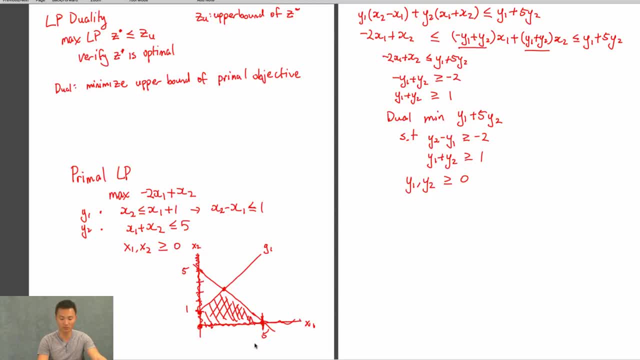 so we have slope of two going up. So we have see, we have contour lines like this, contour lines like this going in, going in right. So it's going to be one of these two, because they're tangent Or I can just check right. 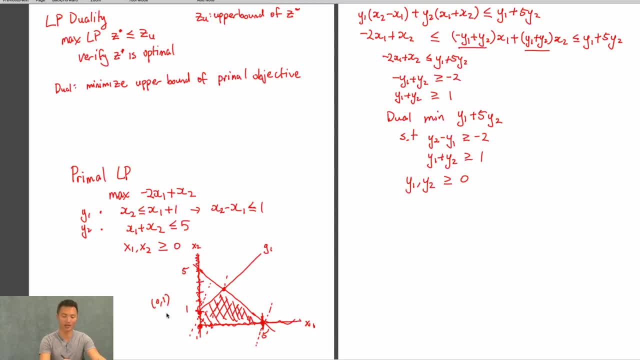 Zero one, we're going to get a objective value of one. Here it's five and zero, So our objective value is actually just going to be negative 10.. So this is my best value, right? So z star is equal to one, and that's using zero and one. 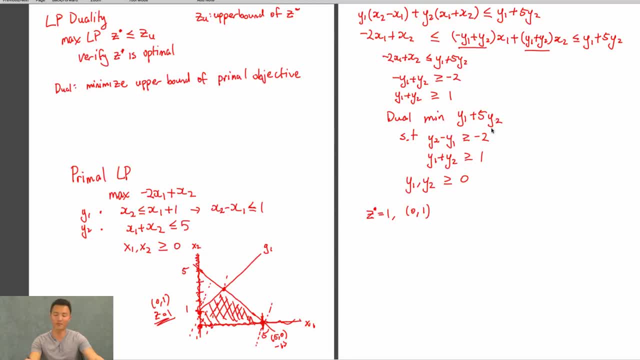 Okay, So what? so what if we minimize the dual? if we minimize dual, we're going to see that. let's see the dual solution for the dual is also going to be one and y. one and y two are going to be one and zero respectively. 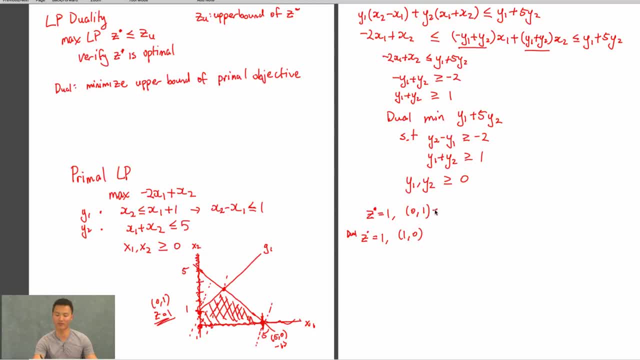 So you can grab this out and you will see that you'll see the same thing. So here we have the optimal y one star and x one star and x two star. Here we have the y one star and y two star. right. 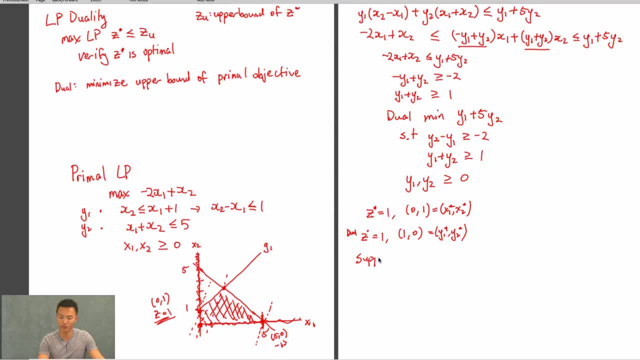 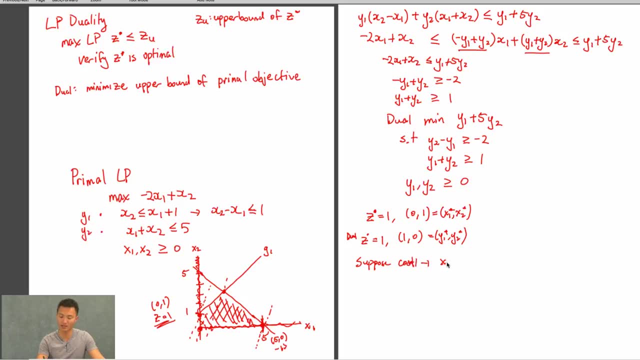 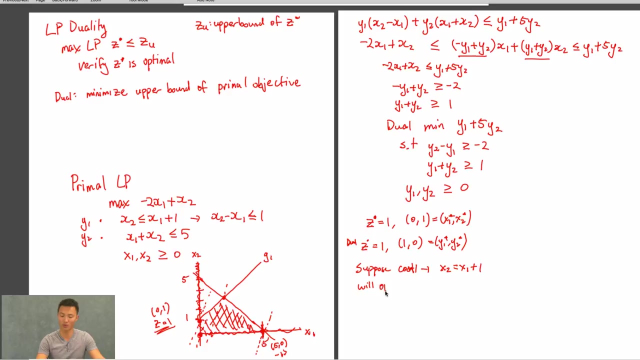 Now here's a question. Suppose that constraint 1 became x2 is equal to x1 plus 1. Will objective optimal objective change? So will the optimal objective change? That's one question. And will the dual change? Now let's take a look at our primal linear program over. 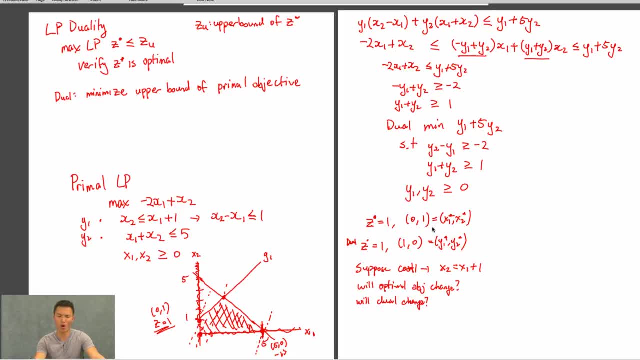 here We see that our objective value is 0 and 1, right, OK. now if our second constraint changes to x2 equals x1 plus 1, like this was originally. so our original feasible region is going to be bigger than the feasible region. 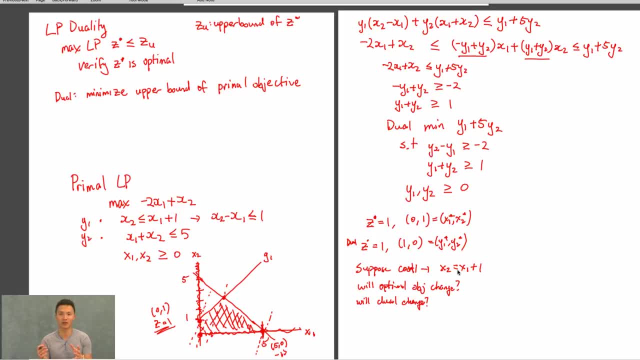 after changing constraint right, Because this is the equality constraint poses a much more restricting area for the feasible region. So we're considering a more relaxed LP and taking it into a more constrained LP. And well, let's look at the optimal decision variables for the more relaxed LP. 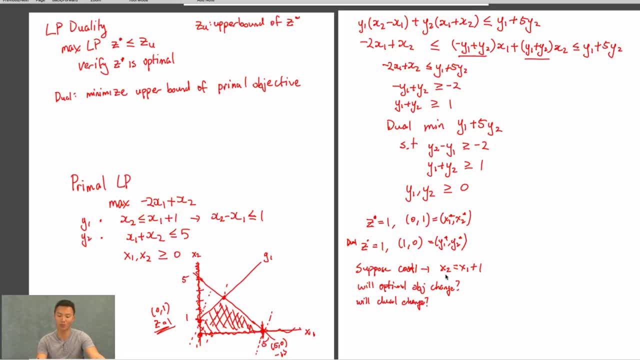 It's going to be 0 and 1, which we can see here. we plug in 0 and 1.. Like, 0 and 1 doesn't change. So what we're saying here is that we're taking the optimal value, that 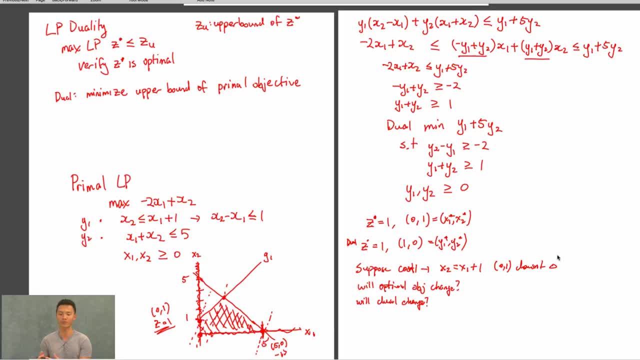 we found the optimal variables that we found and the more relaxed LP is not going to be violated. It's not going to violate any constraint. when we make that LP more constraining, Then this must also have to be optimal for the more constraining LP.